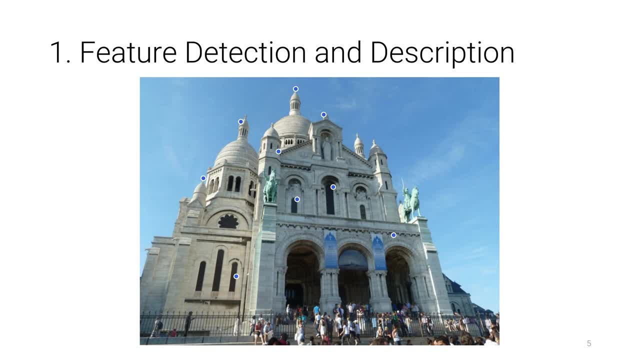 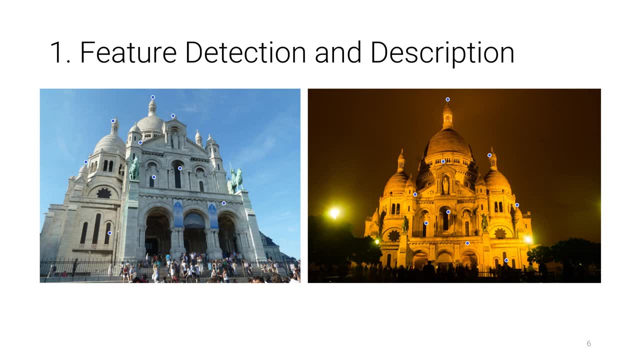 Usually located on distinctive structures such as corners. This process is repeated for all images in the scene and one computer features the scriptor for each key point, which encodes the appearance information of its local neighborhood. Each key point is matched to its most similar counterpart in each of the other images. 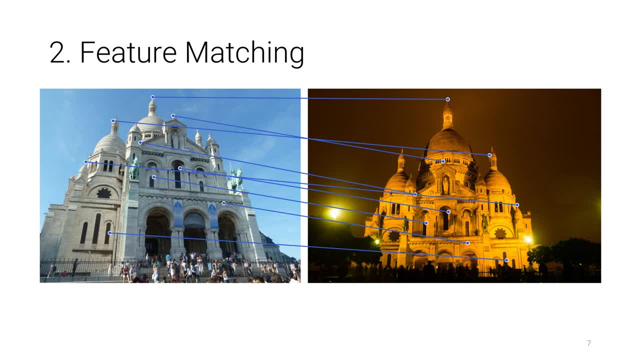 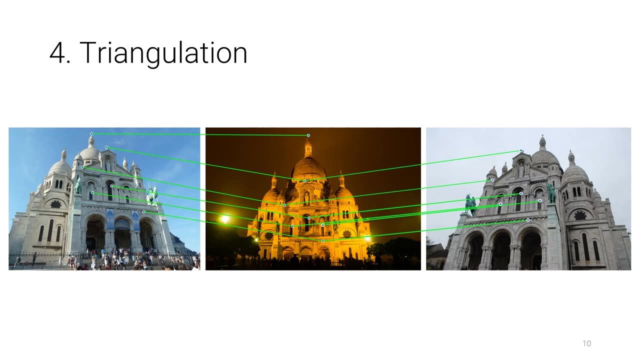 Since descriptors only encode local information, this can yield a large number of incorrect matches. Using epipolar geometry, inverted matches can be filtered at an early stage. The matches graph can be constructed by matching other images in the same time. the scene and matches across multiple views are called tracks. In the next step, tracks are 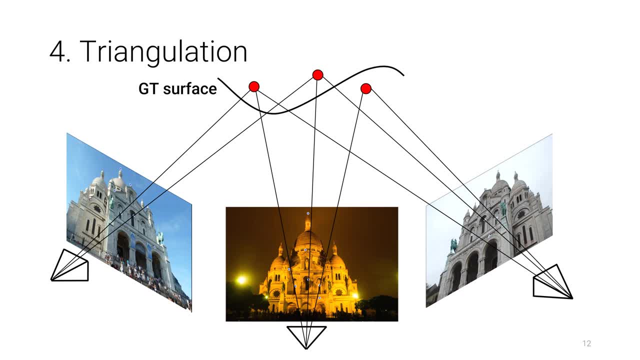 triangulated to obtain 3D points, and this process is repeated for each track in the matches graph. While both 3D structure and camera poses are refined by minimizing the 2D reprojection error in a global optimization problem called bundle adjustment. While the SFM pipeline is robust, it 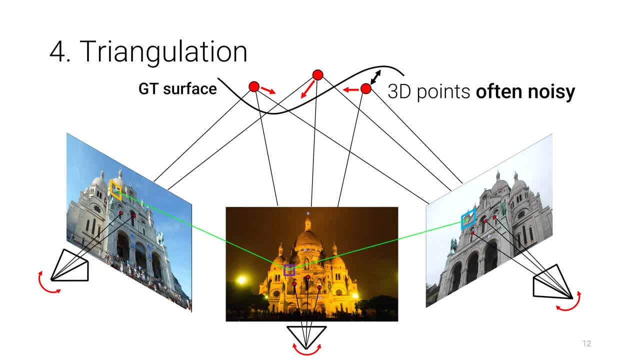 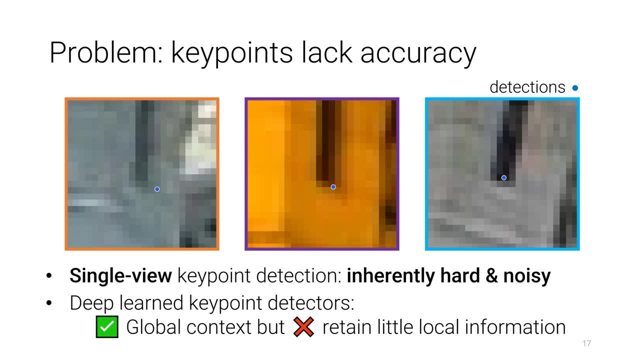 often yields noisy 3D point clouds. Let's have a look on why this happens. in a given track, Key points are detected for each image separately and need to be matched globally. Thus they are not perfectly aligned over multiple views. This problem is compounded in recently learned feature detectors, which are designed to encode. 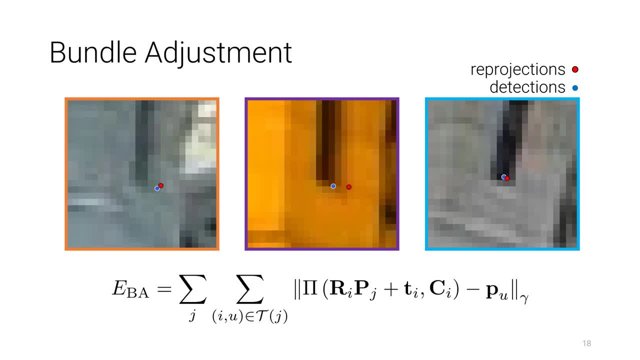 global context at a lower resolution. This noise has significant impact on the quality of the resulting 3D model because standard SFM pipelines apply bundle adjustment with a geometric reprojection error. Here the 2D projection of a 3D point in its observing image. 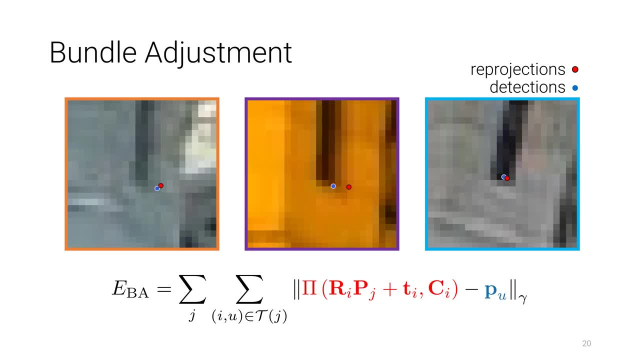 is a 3D projection of a 3D point in its observing image Compared to the noisy location of its corresponding detection, and their 2D distance is minimized. Noisy initial detections will therefore propagate through the entire SFM pipeline and result in noisy 3D points and camera poses. 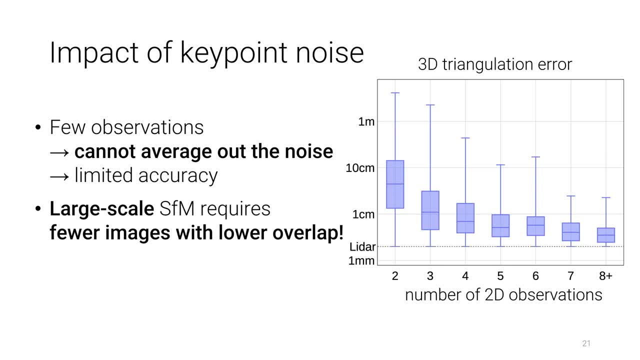 By increasing the number of images which observe the same 3D point, this error can be reduced, Though in many cases this is infeasible, since it requires a large view overlap. Scaling SFM to large scenes, on the other hand, is made easier if few observations are redundant. 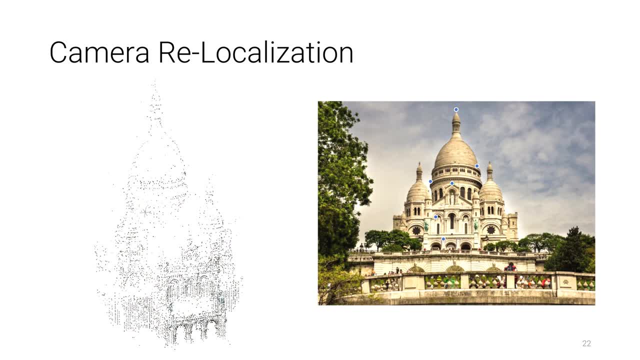 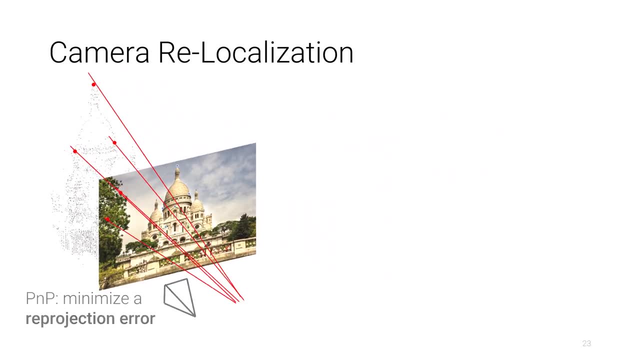 Noisy keypoints also impact subsequent tasks, such as camera relocalization, where we estimate the 6dof pose of an unknown image with respect to an existing 3D model. Detections in the query image which are just a few pixels off can result in large pose errors. 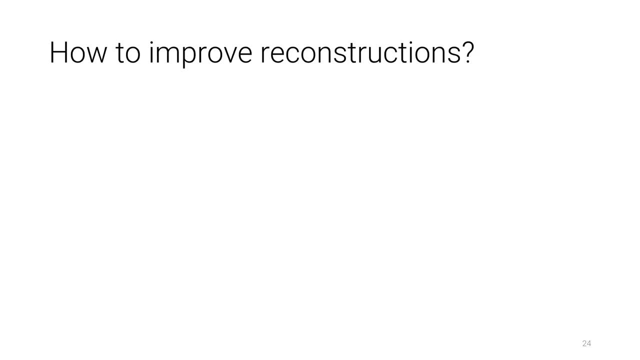 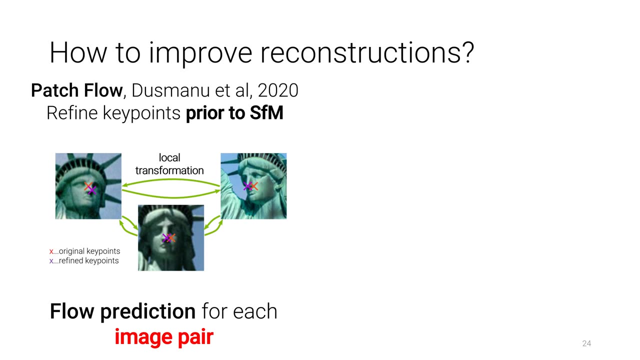 The same applies to noisy 3D models To improve reconstructions. recent methods like patch flow aim to refine the initial detections by estimating the flow of local image patches. While this is shown to be significantly more accurate, it requires expensive flow predictions for each image pair. 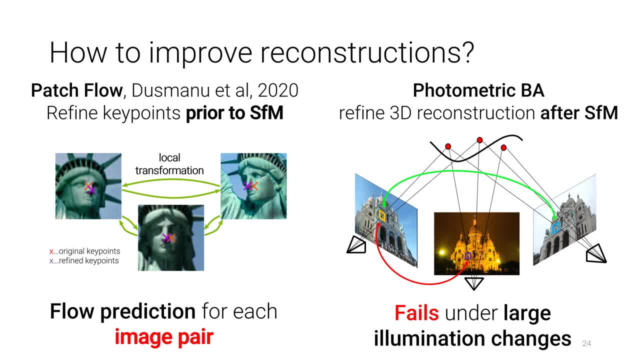 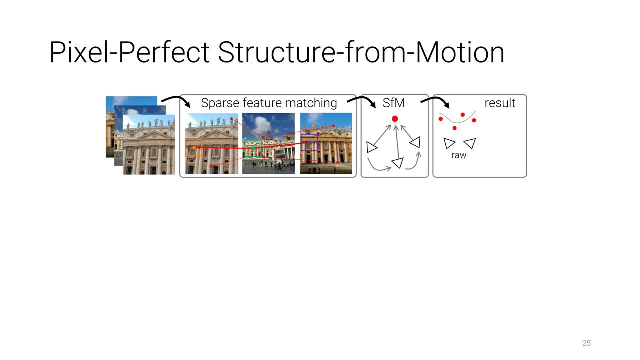 Photometric bundle adjustment uses appearance information to refine the 3D model after SFM by minimizing the appearance difference of local patches, but fails under large illumination changes such as day and night images. We propose pixel perfect structure for motion which improves both initial detections prior to SFM and the final 3D scene. We start by feeding each image. 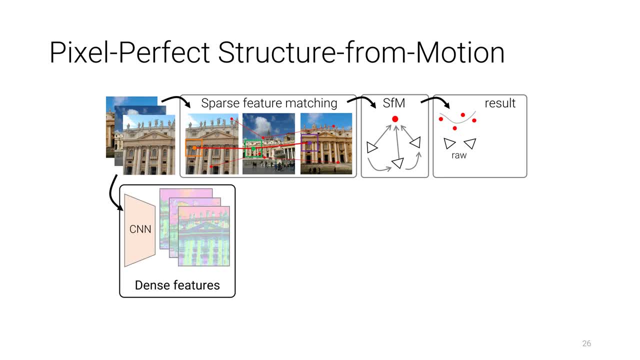 a convolutional neural network to obtain dense, high dimensional feature maps. In feature metric keypoint adjustment we align deep features on the tentative matches graph to refine initial detections jointly over multiple views by direct optimization. The refined keypoints are forwarded to the standard SFM pipeline to estimate a 3D reconstruction. In feature metric bundle adjustment. 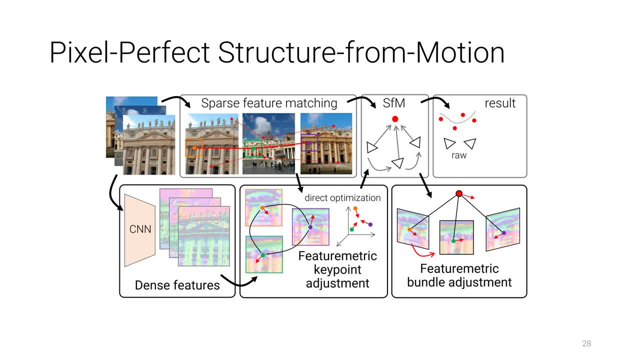 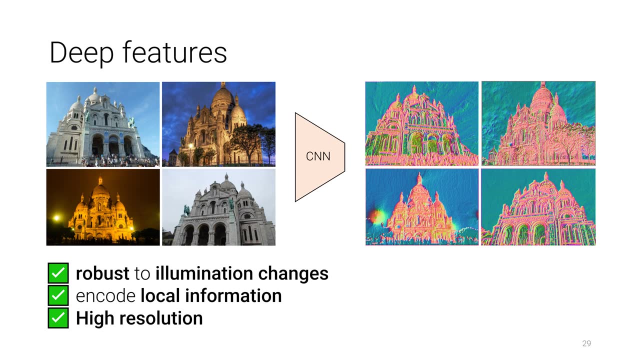 we propose to refine both poses and 3D structure globally using the same deep features. This direct optimization pipeline improves both accuracy and completeness of 3D models. The system requires deep features which are both robust to illumination changes and encode local appearance information in high resolution With locally smooth and accurate feature metric cost. 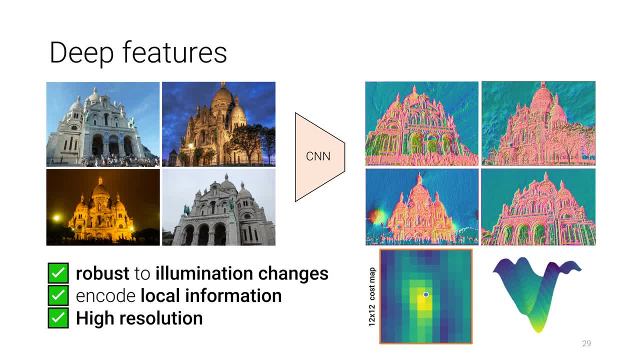 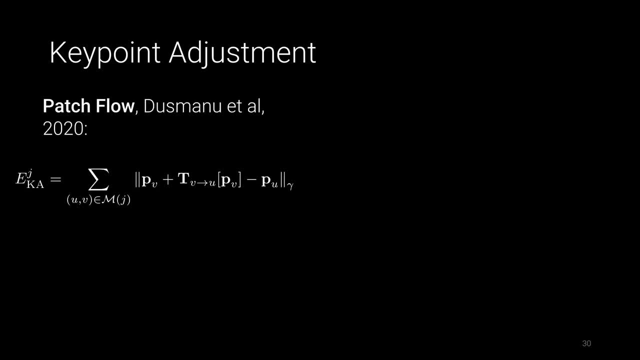 functions around match detections. even coarse priors can converge accurately. The next step is keypoint adjustment, where the current state of the art approach is patch flow. We estimate a flow field between matched image patches using a CNN and compares the flow adjusted keypoint to its match correspondence, minimizing the distance between 2D points. This optimization 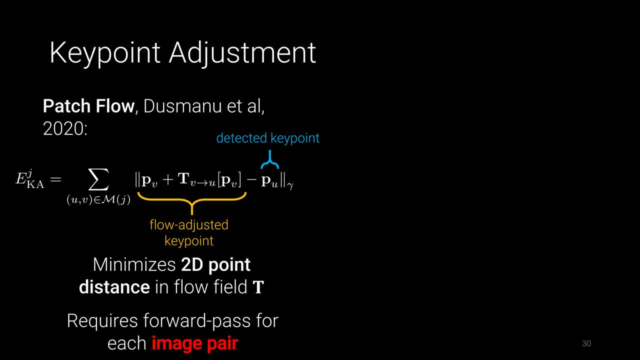 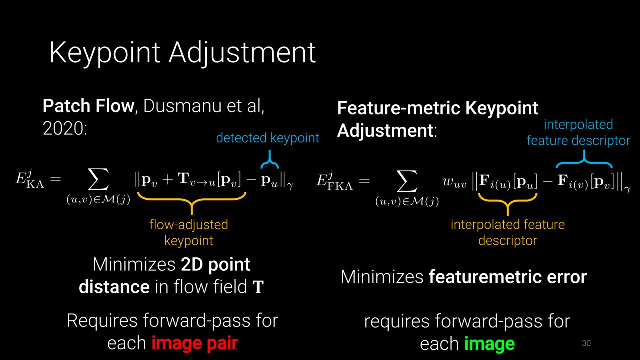 has quadratic complexity in the flow T. Our feature metric keypoint adjustment directly minimizes the difference between interpolated descriptors at keypoint locations. In contrast to patch flow, the gradients in the deep features implicitly define a flow field and we therefore only need one forward pass for each image. In practice, we take the keypoints of a match track. 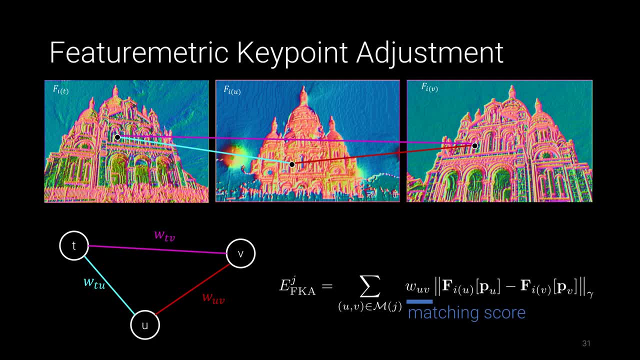 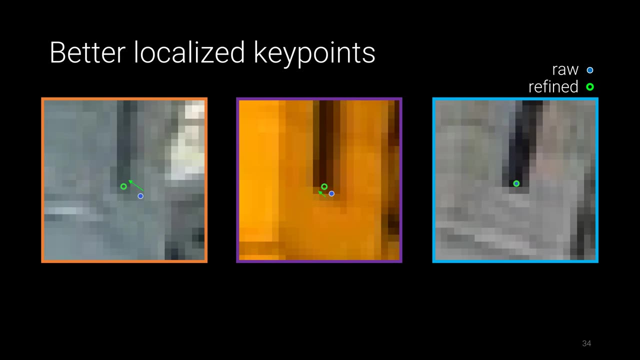 and build a graph with edges weighted by the matching score. The graph is then optimized by minimizing the feature metric error along each edge and we fix the keypoint with the highest aggregated matching score to avoid drift. Feature metric keypoint adjustment results in better localized features across multiple views, effectively reducing the noise of keyboard detectors and. 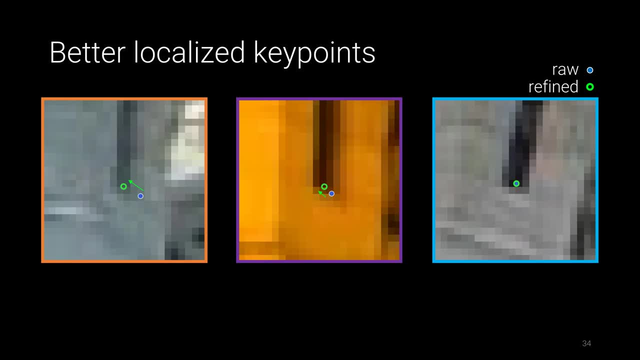 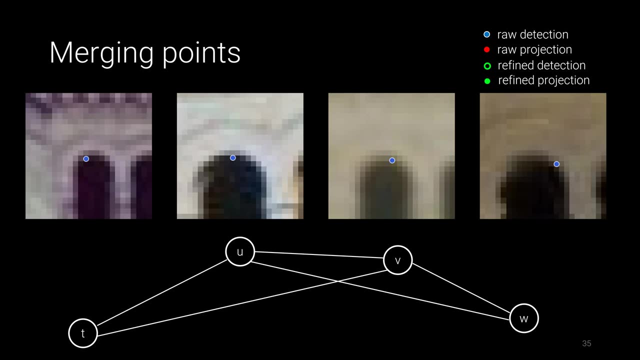 the overall number of triangulated points. in the reconstructed model We find keypoints can also effectively increase the track length of triangulated points. Here we have a track where all four features are matched together, but because of noisy keypoints ColMap fails to merge points during triangulation and instead creates two separate, smaller tracks. 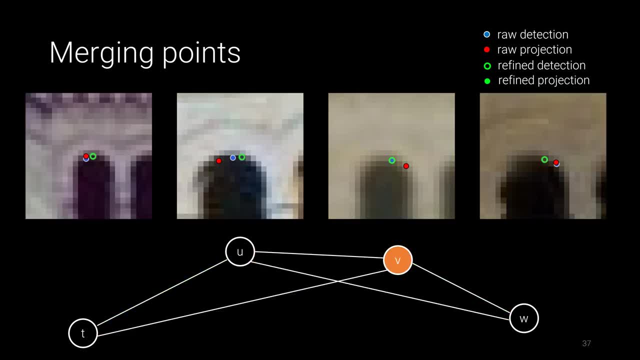 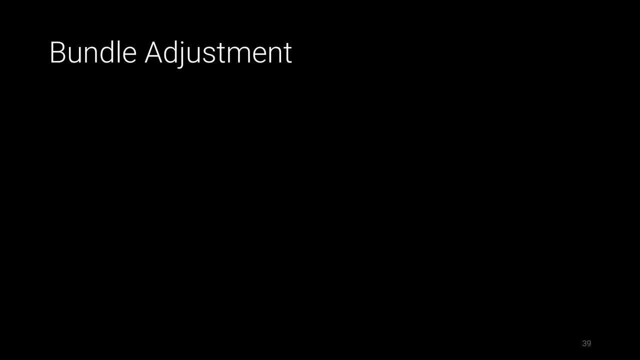 with large reprojection error. Feature metric keypoint adjustment reduces this detection noise in the graph jointly and ColMap is then able to correctly triangulate the matches to a single, more robust 3D point with larger track length and smaller reprojection error. The second proposed refinement is in bundle adjustment. In classic SFN one usually minimizes 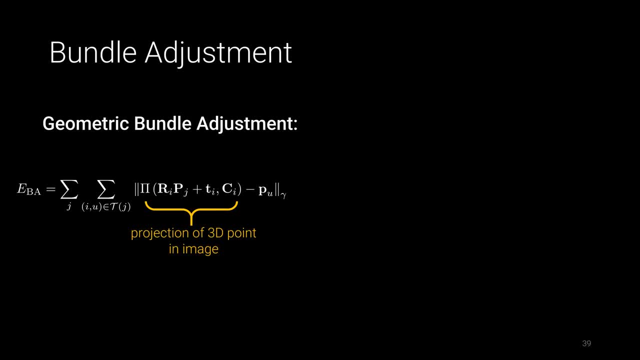 the geometric reprojection error between the projection of a 3D point in an image and the corresponding keypoint location. While this global adjustment is robust throughout layers, it does not use any appearance information. Feature metric bundle adjustment interpolates deep feature maps at a 3D point projection. 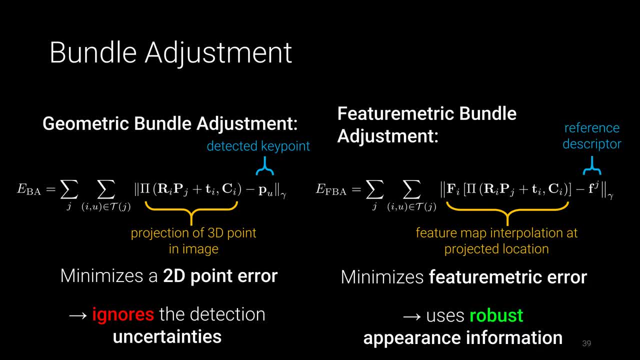 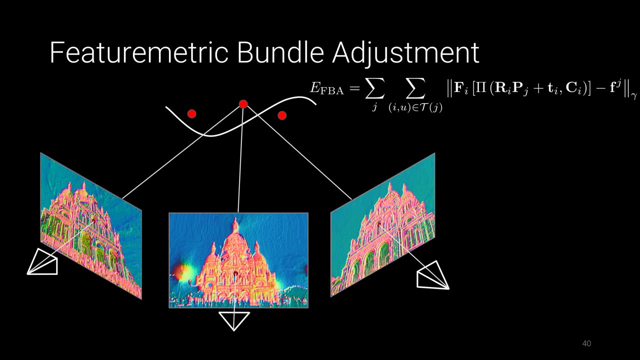 and compares it to a fixed reference. Both poses and 3D points are globally adjusted to minimize the feature metric error. This direct optimization uses robust appearance information contained in the deep features. It takes as input a sparse 3D reconstruction obtained from structure from motion To estimate a reference descriptor for each track. 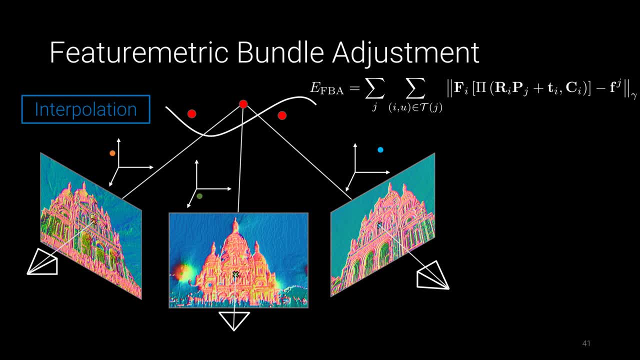 we first interpolate the feature maps at their current reprojection locations. Compute the robust mean using iteratively weighted least squares. The interpolated descriptor most similar to the robust mean is selected as the reference for this track and remains fixed during optimization. The local feature metric. 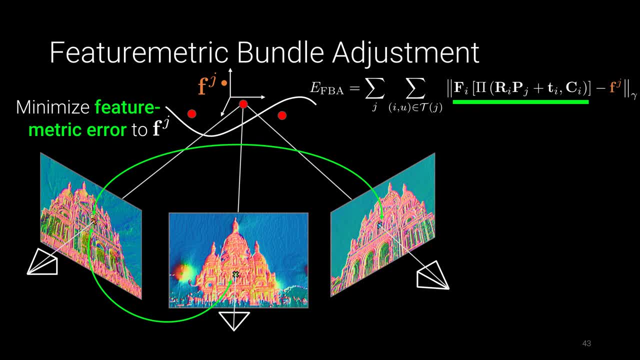 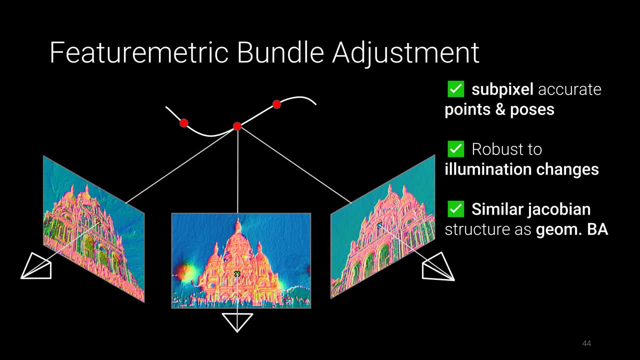 gradient at reprojected locations towards the robust reference allows to globally refine both 3D structure and camera poses. This results in a sub-pixel accurate 3D model, while the pipeline remains robust to real-world challenges such as illumination changes. Note that the Jacobian sparseness pattern is similar to geometric SFM and does: 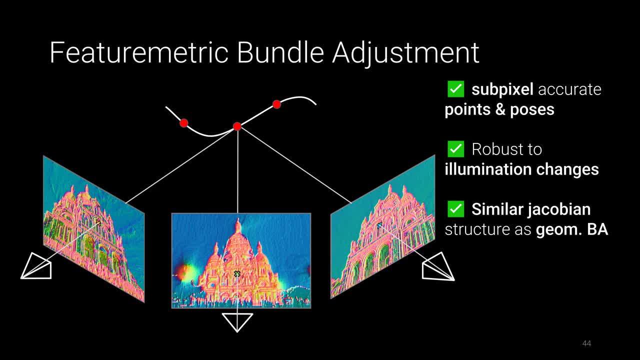 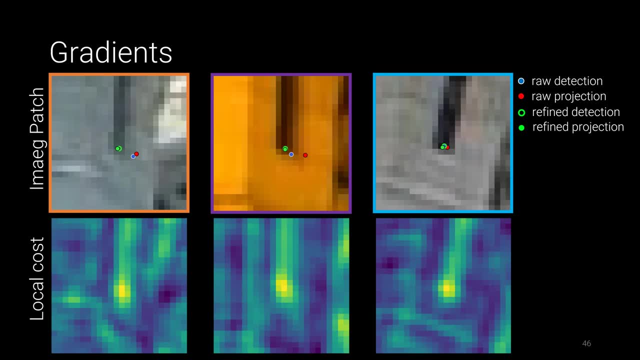 efficient schemes like the skirt complement track apply. The re-fine reprojections are much better localized compared to the geometric counterpart. Feature metric BA allows to further reduce noise over key-point adjustment by utilizing geometric constraints. The obtained gradients towards the robust reference are locally smooth, allowing large convergence from coarse priors. 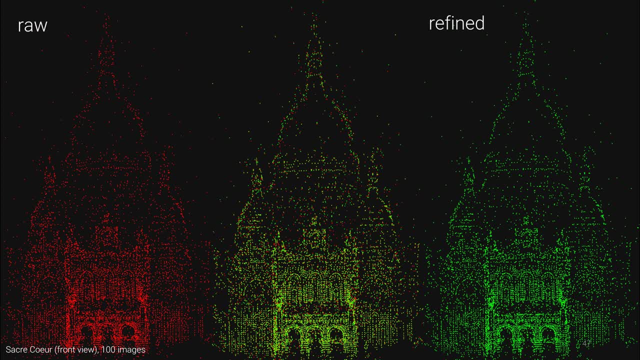 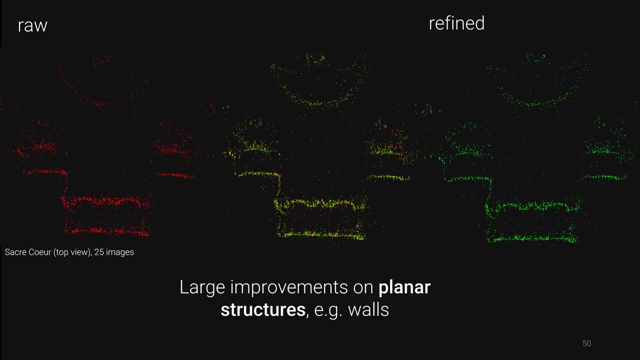 Our method can reconstruct local geometries such as the horizontal lines on this tower, but also large elements like the outside of the main dome. Textured surfaces like arches and monuments with fine details can be recovered using pixel-perfect structures of motion, And from a top view one can see that especially planar. 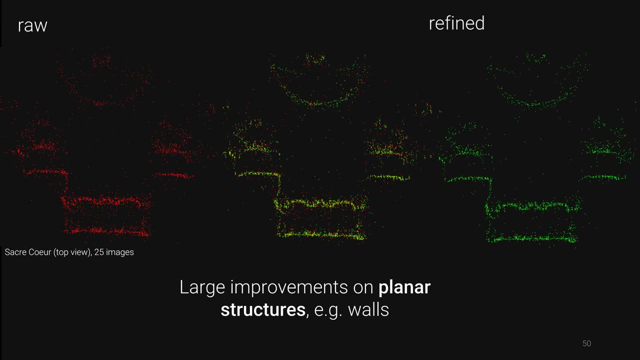 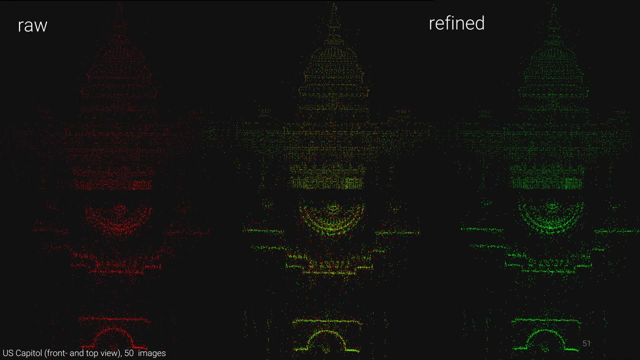 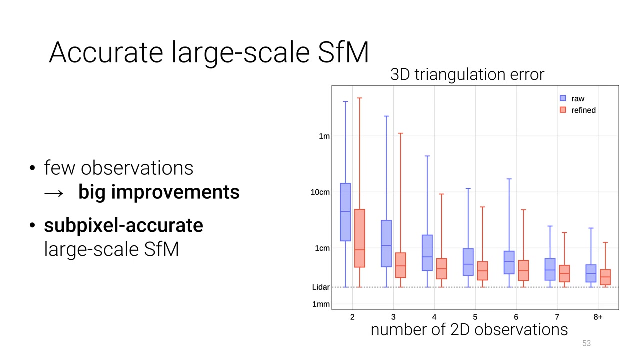 structures like walls are significantly improved, even on smaller scenes. Here is another example of the US Capitol, where our system triangulates many more points which are also more accurate. The proposed pipeline yields close to lighter accuracy and greatly improves points with only a few observations enabling subpixel accuracy in. 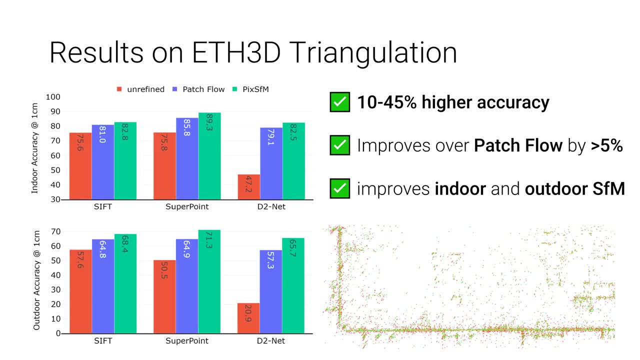 large-scale SFM Both on indoor and outdoor scenes. pixel-perfect structure for motion outperforms both ColMap and PatchFlow on the ETH 3D triangulation benchmark. Especially learned features like SuperPoint or Detonet benefit from our refinement. 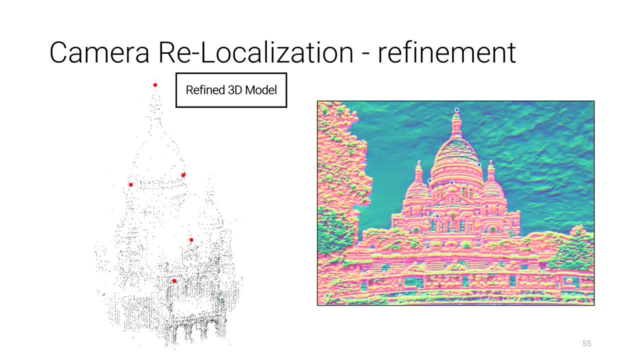 We also compare our method in camera relocalization. We propose a feature metric refinement strategy. After finding 2D-3D correspondences, we extract a reference descriptor for each 3D point and refine the key points in the query image by minimizing the feature metric error to the 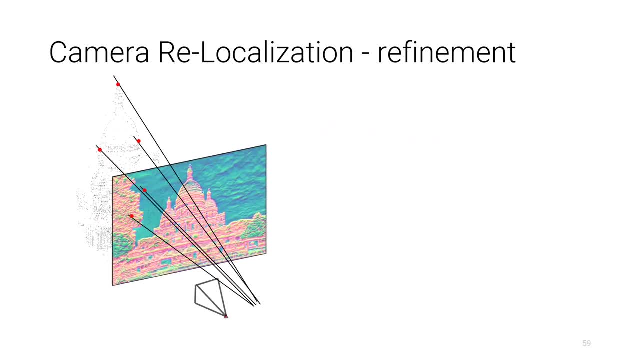 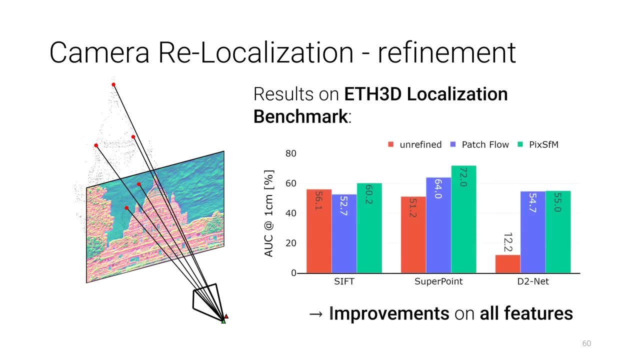 reference. The perspective endpoint algorithm is used to estimate a rough prior for the camera pose, which is again refined by aligning deep features. We evaluate the localization accuracy on the ETH 3D dataset. The method clearly outperforms PatchFlow on both.